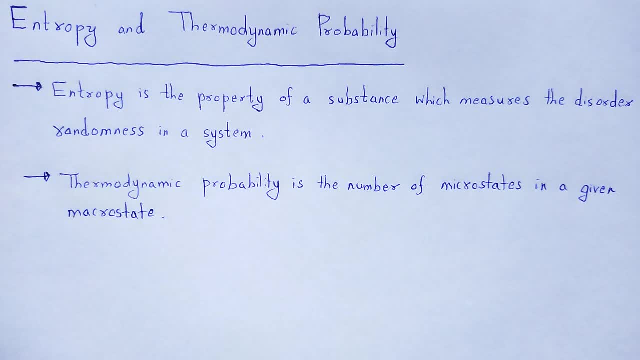 Hello students, good time to all. I am Chandan Kwan Pradhan. Welcome to YouTube channel Chandan Physics. In this video we are going to discuss entropy and thermodynamic probability. Let us begin. Entropy is the property of a substance which measures the disorder or randomness. 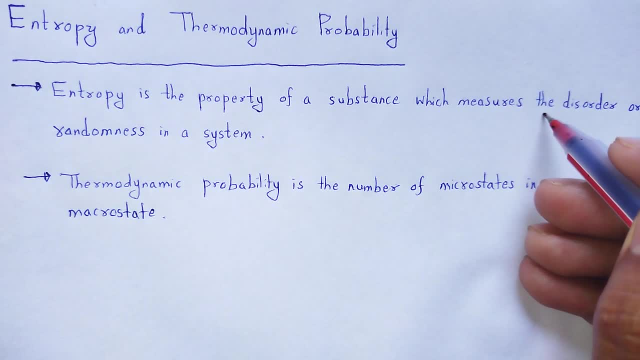 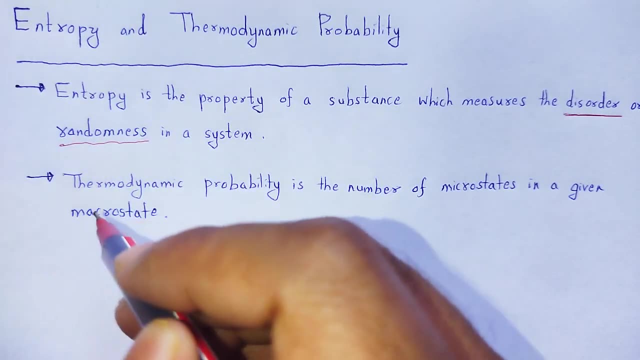 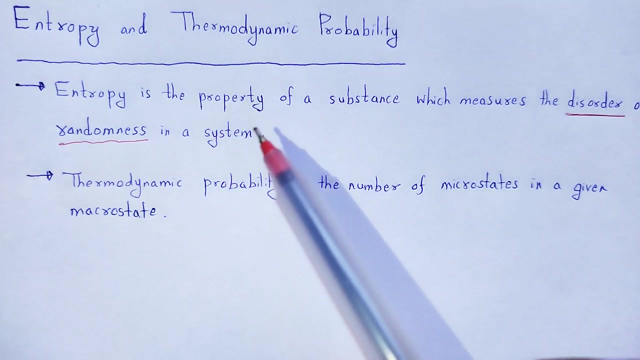 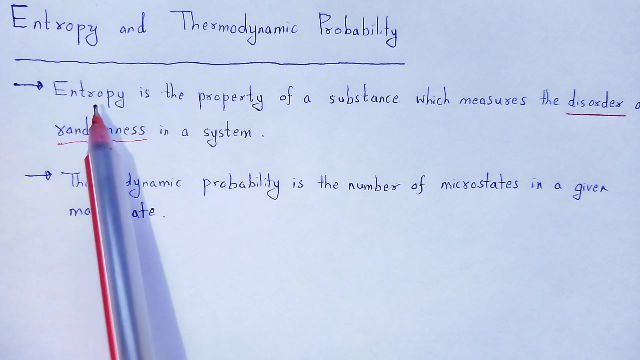 in a particular system. The measure of disorder and randomness, The concept of entropy, has been introduced to describe the natural tendency of the system, That natural tendency to attain most probable macro state. What is the state and the macro state? We have already discussed Entropy. is a state function. What? 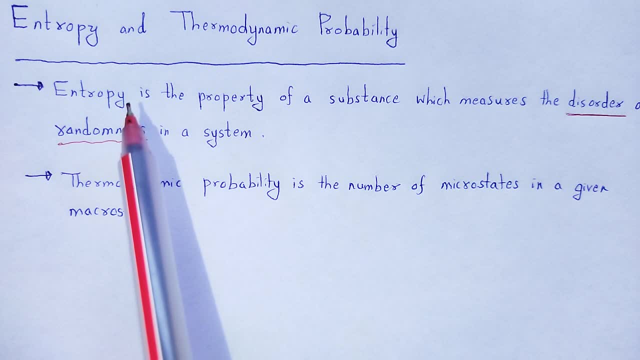 is the state function. A state function for a particular physical quantity is defined as that: the physical quantity initial and final condition, not to the intermediate situations. Entropy depends on the initial state and final state not within that of intermediate states. So entropy is a state. 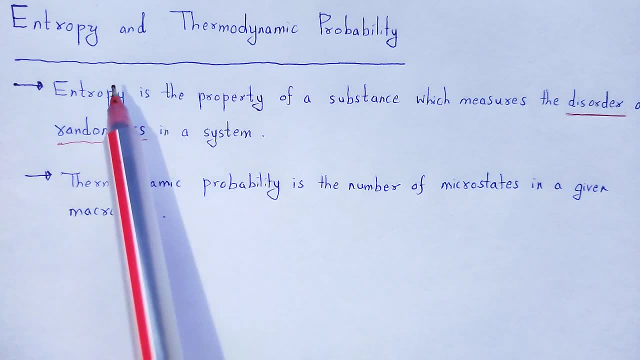 function and it is additive in nature, Entropy of a number of systems can be added. If we consider two systems- one system have entropy S 1 and another have entropy S 2, then the total entropy of that system is equal to S 1 plus S 2.. 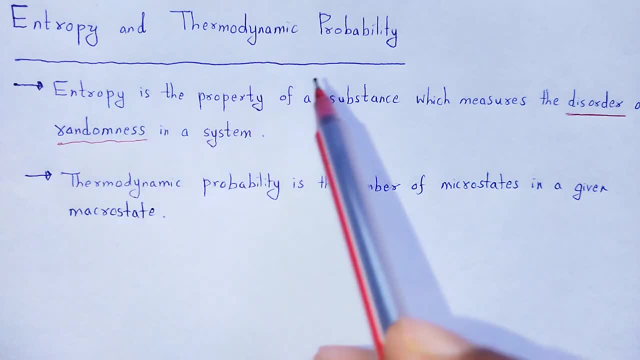 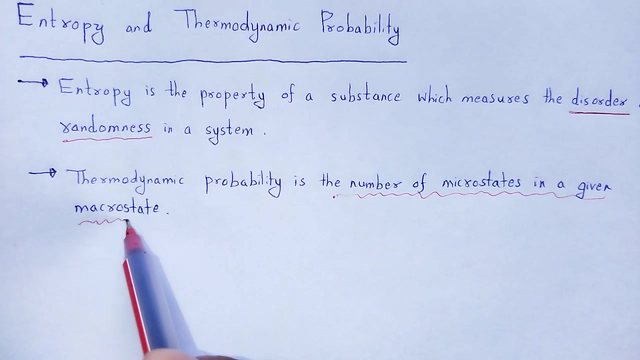 Entropy is additive in nature. Next, thermodynamic probability. Thermodynamic probability is the number of microstate in a given macrostate. What be the number of microstates present in a given macrostate is called thermodynamic probability, or we call it as frequency. 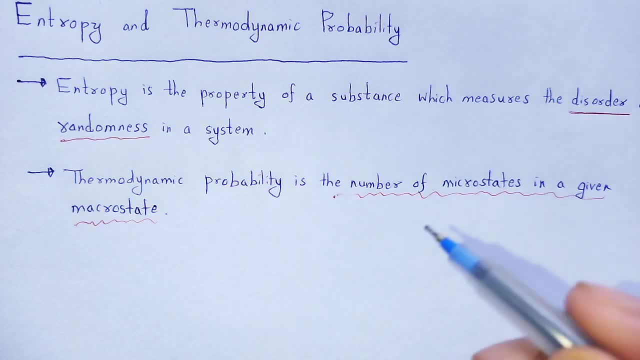 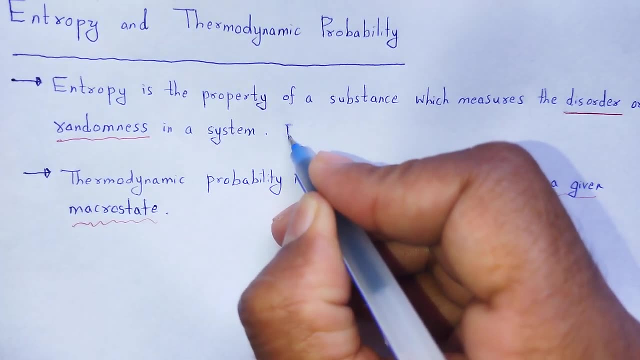 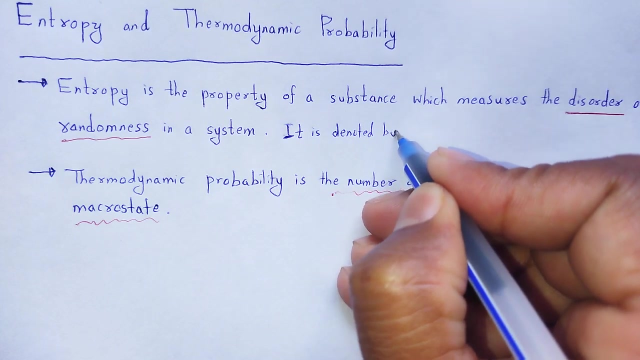 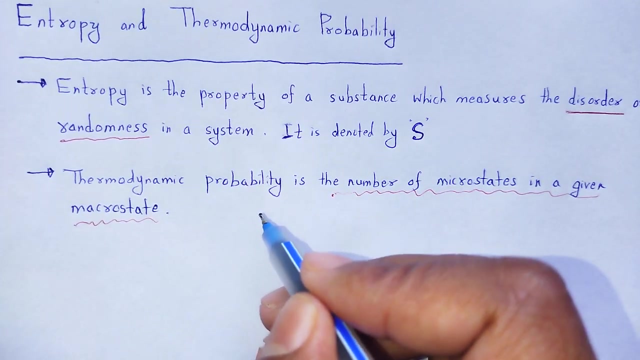 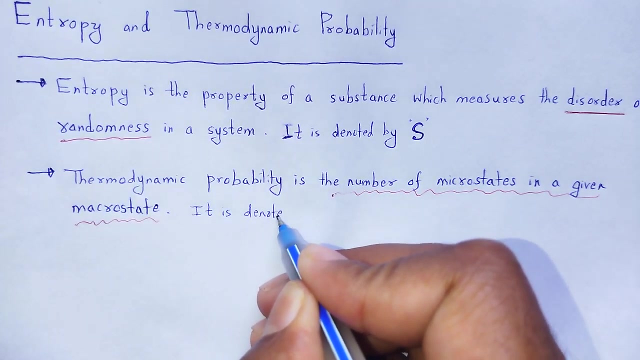 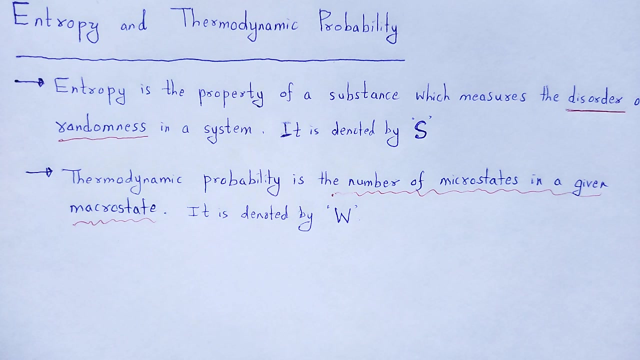 The entropy is denoted by the letter S. Thermodynamic probability is denoted by the letter W, the letter W. Now we have to derive what be the relation in between entropy and thermodynamic probability, Which one is called The statistical definition. 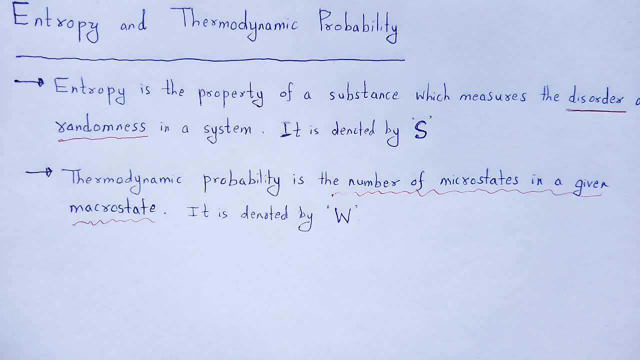 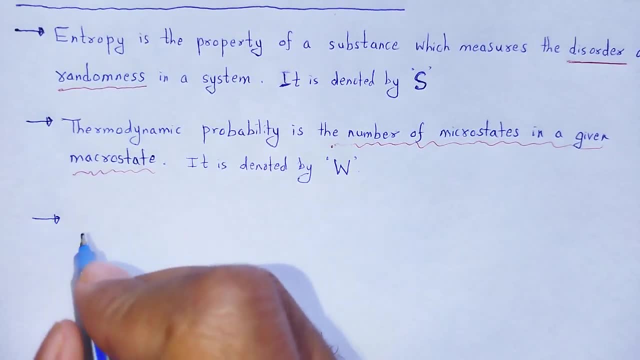 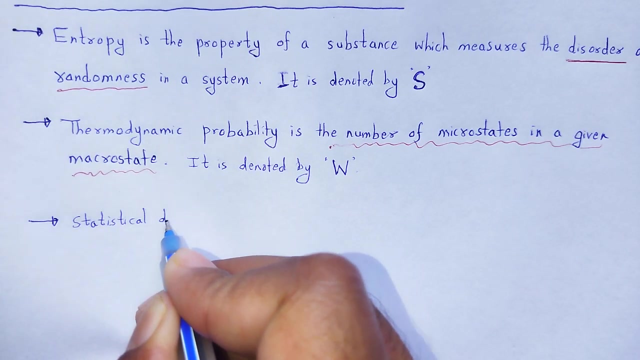 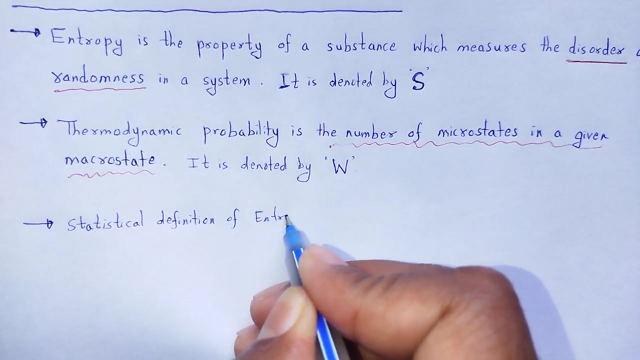 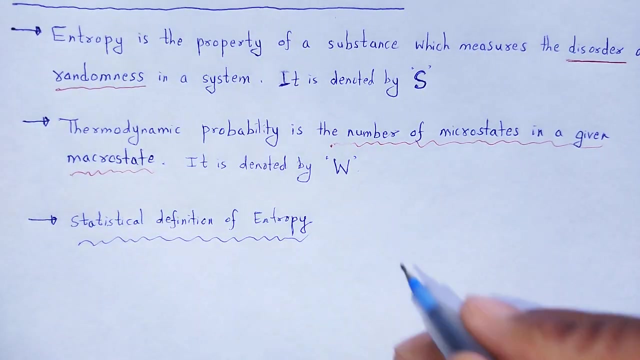 of entropy. Statistical definition of entropy, or we call it as …. The entropy is denoted by the number of eight forms. For example, you have to derive the F of S. you have to derive the F of S. The entropy is denoted by the number of 6 elements. 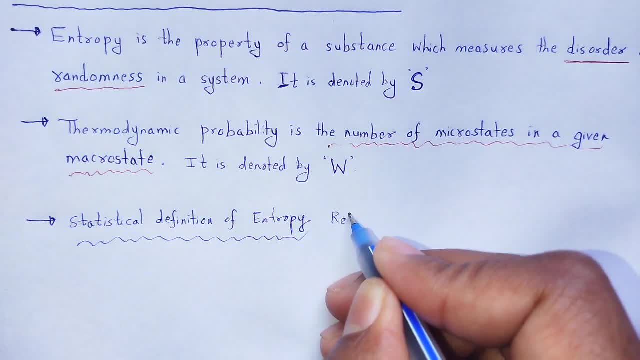 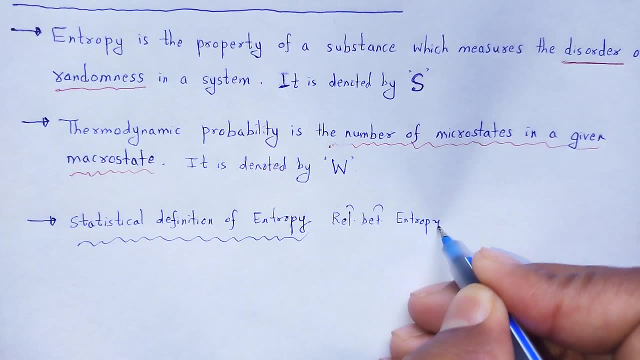 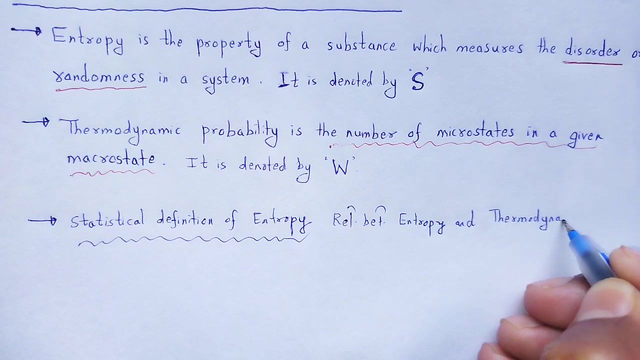 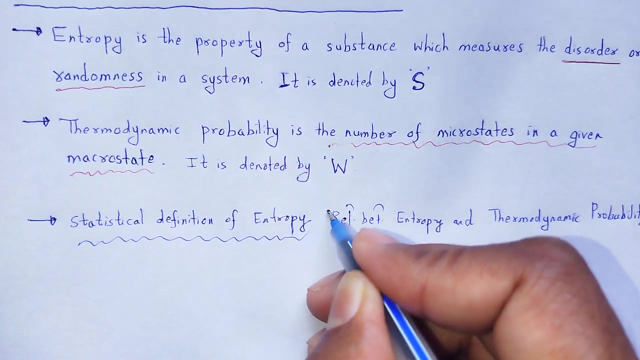 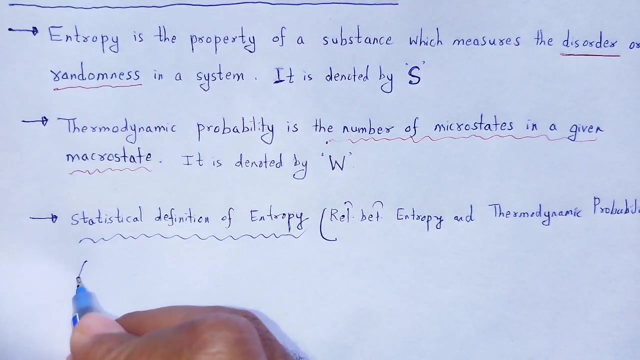 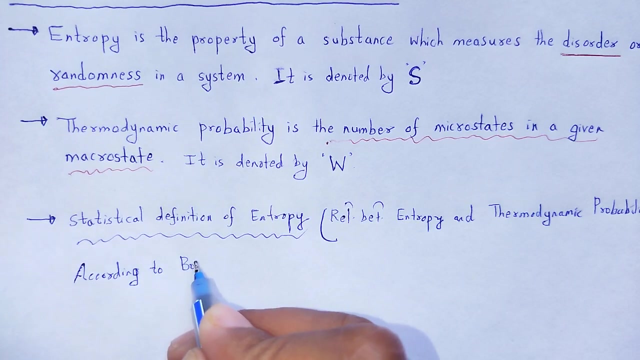 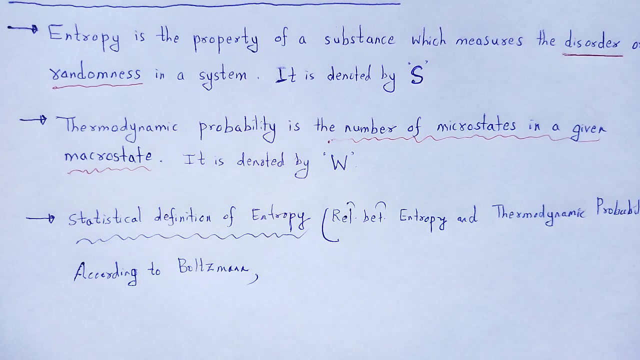 The entropy is denoted by the number of 8 elements. relation between entropy and thermodynamic probability According to Boltzmann. Boltzmann observed that at absolute temperature- absolute temperature means at 0 degree Celsius- the system has entropy 0 and its thermodynamic probability 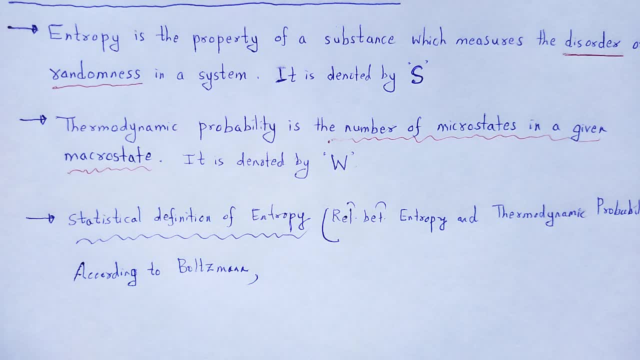 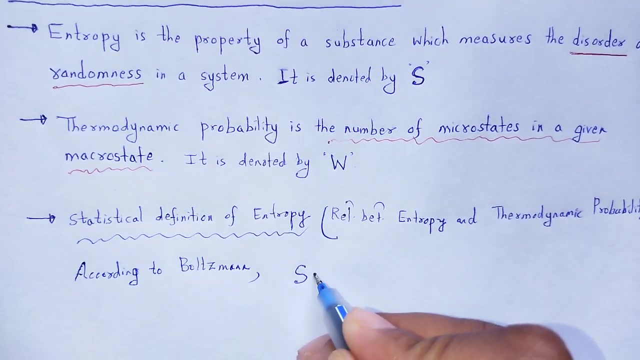 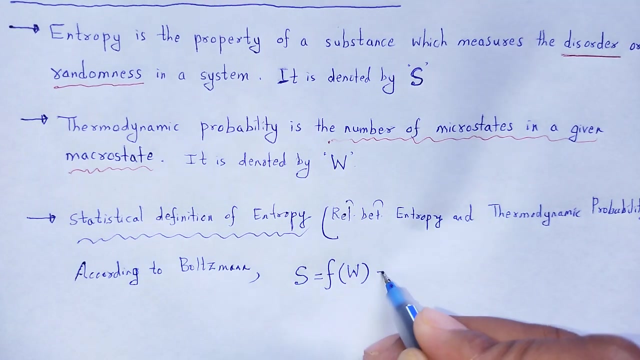 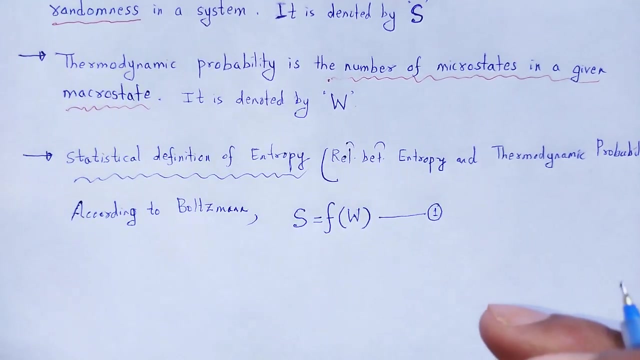 is 1.. So he takes a concept that how entropy of a system is the related to the thermodynamic probability. So he confirmed that entropy is a function of thermodynamic probability. that equation number 1.. Let me take a system. 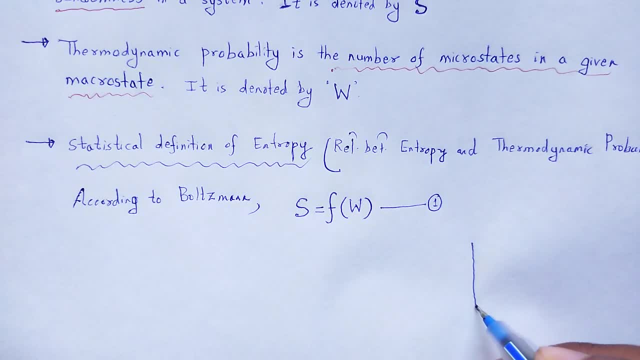 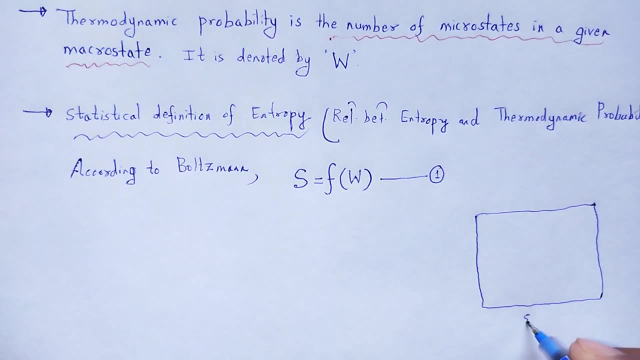 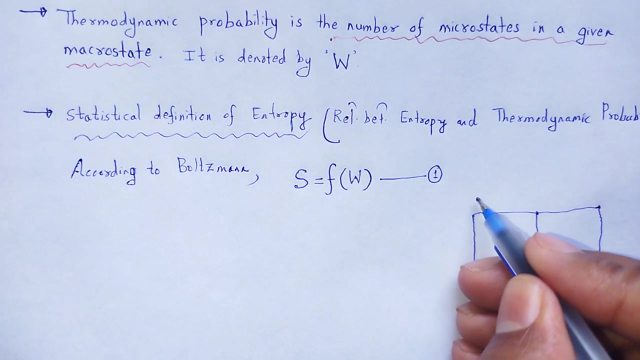 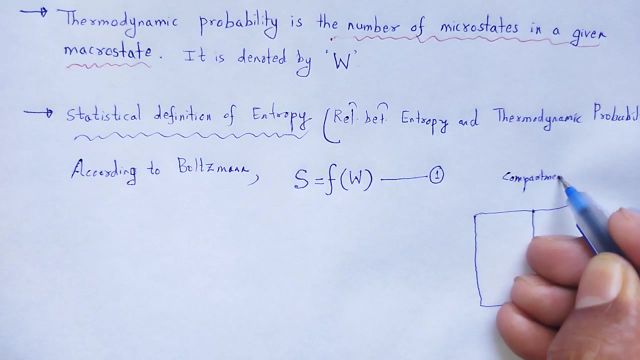 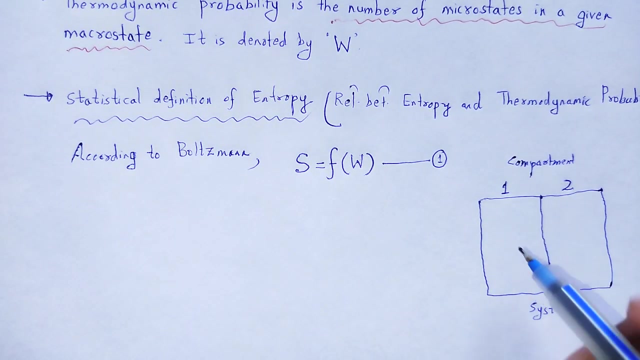 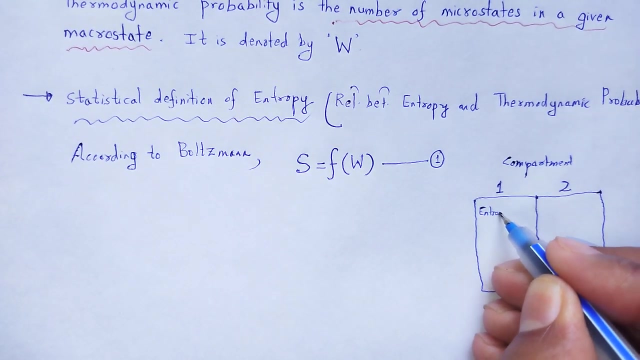 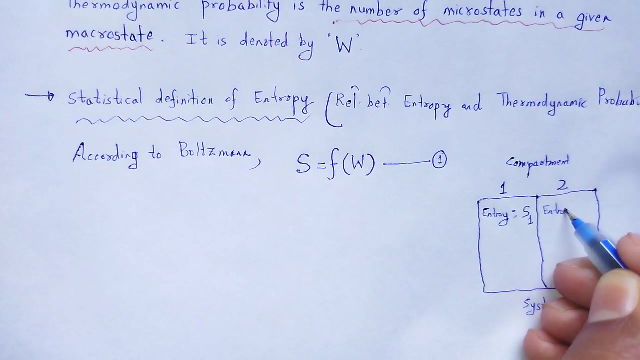 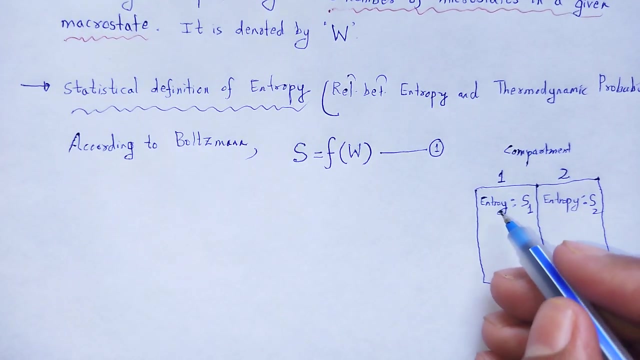 So this system, it has two compartments. This is compartment 1, that is compartment 2.. as entropy, the entropy as S 1, here the entropy of compartment 2, S 2 and the thermodynamic. 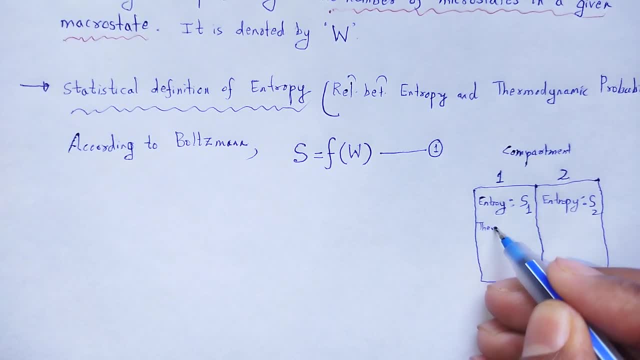 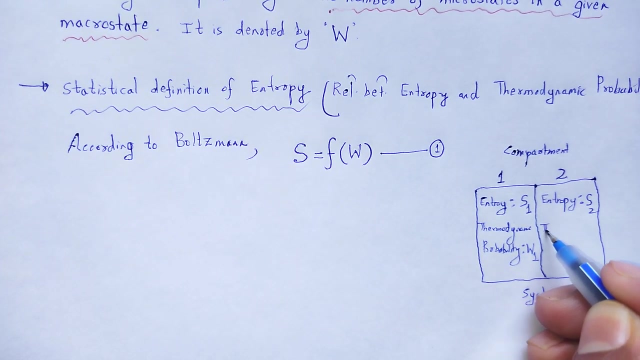 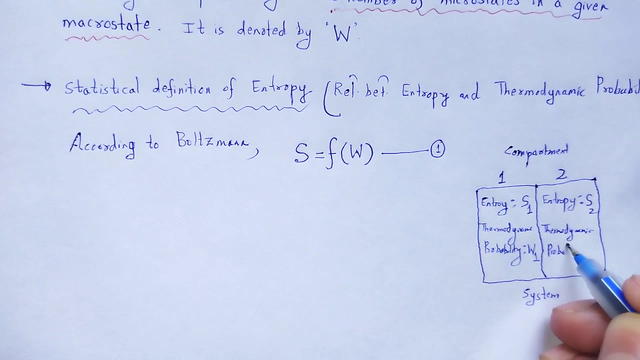 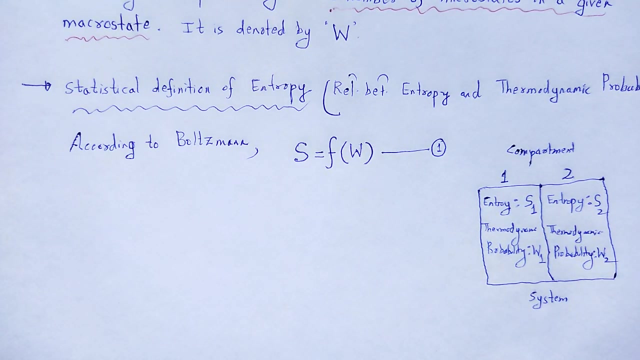 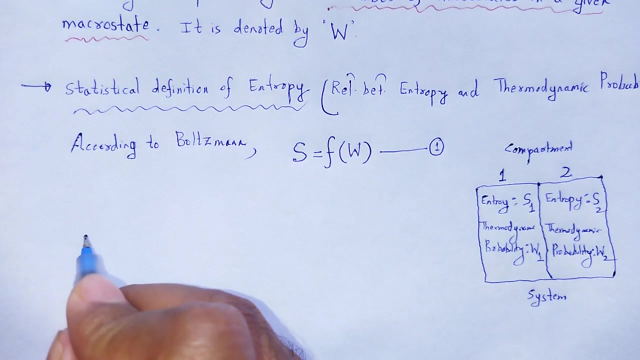 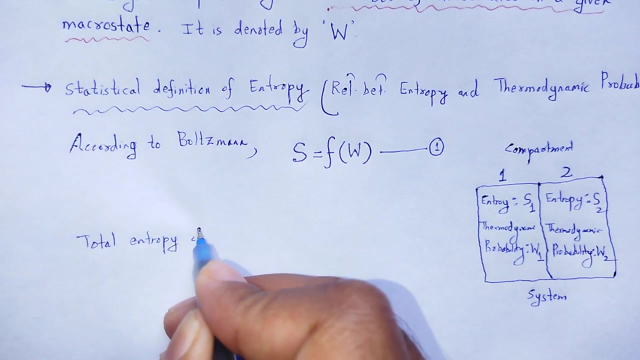 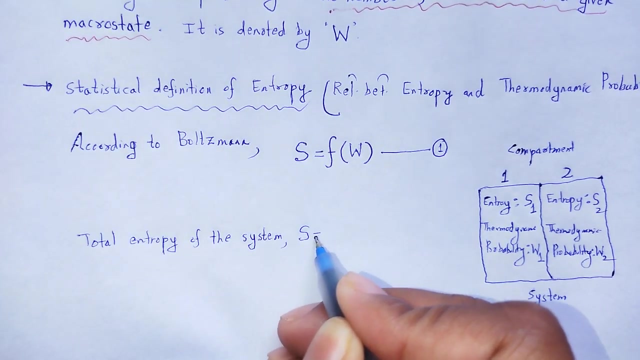 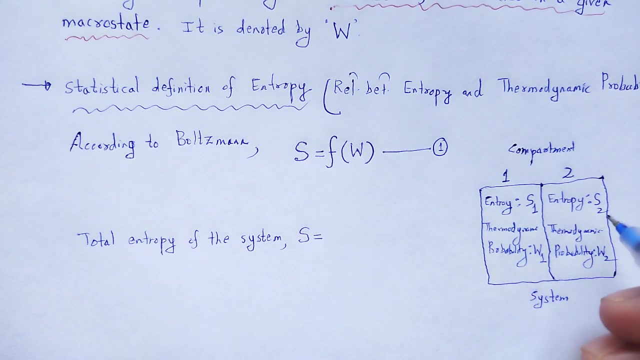 probability. thermodynamic probability here: let W 1, compartment 2, the thermodynamic probability, let W 2.. So total entropy of that of system, total entropy of the system S is equal to entropy of compartment 1 and entropy of compartment 2.. 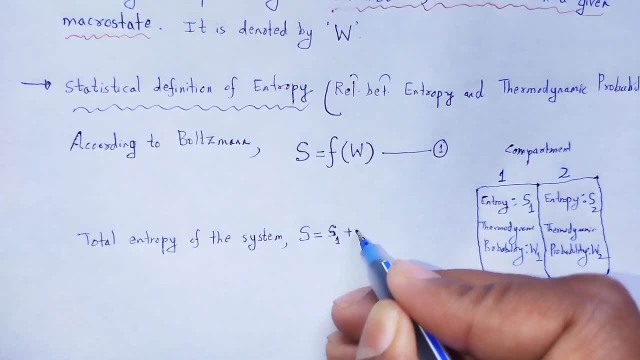 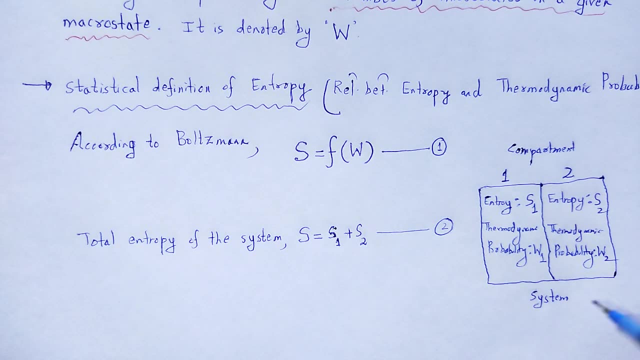 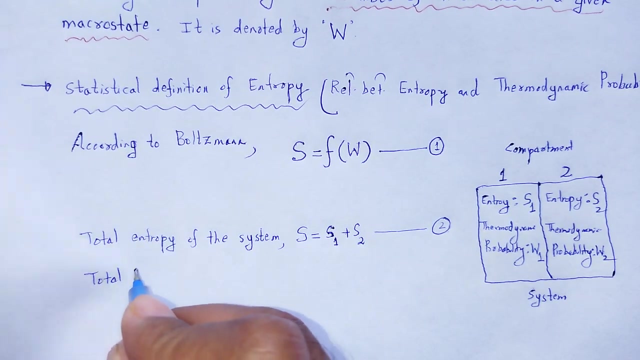 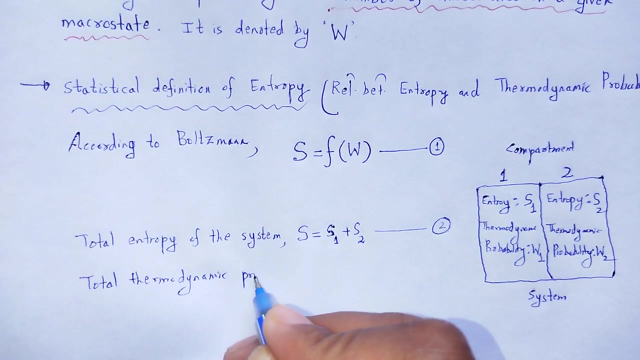 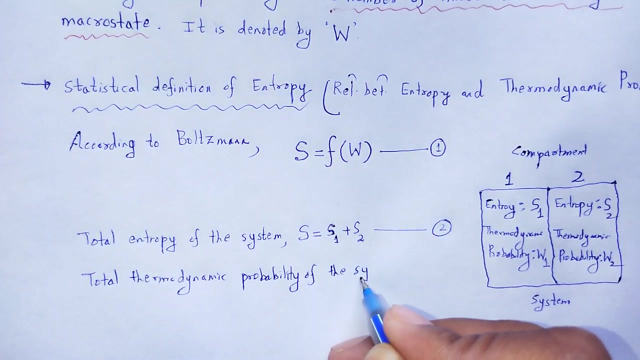 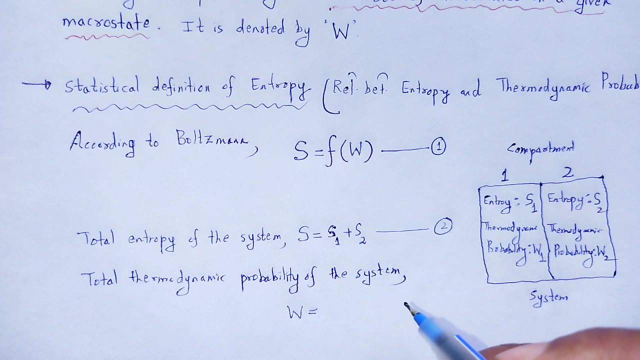 of compartment 2, S 1 plus S 2, equation number 2.. And total thermodynamic probability of the system. total thermodynamic probability of the system, that is, W, is equal to. according to the definition of thermodynamic probability, the total thermodynamic probability is equal. 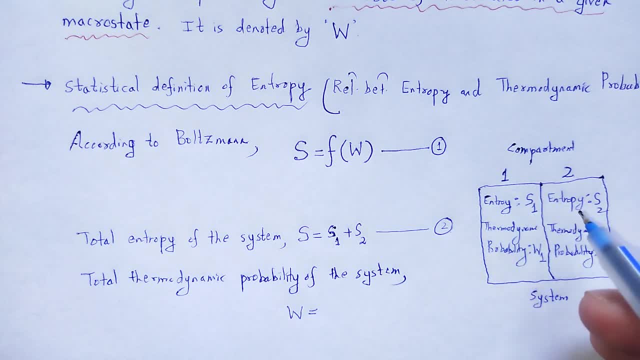 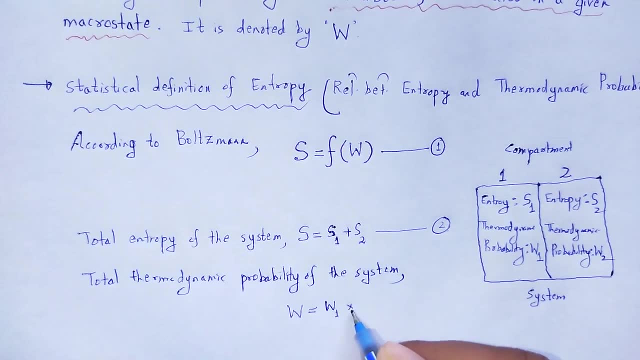 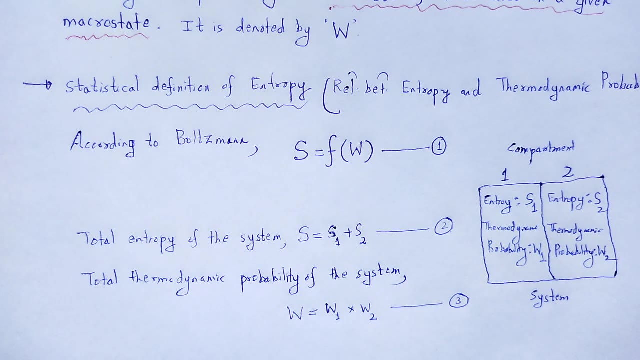 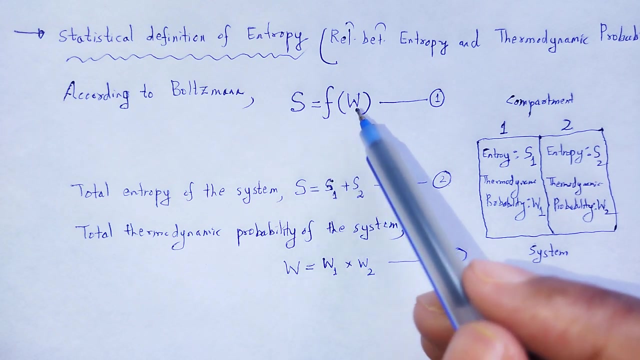 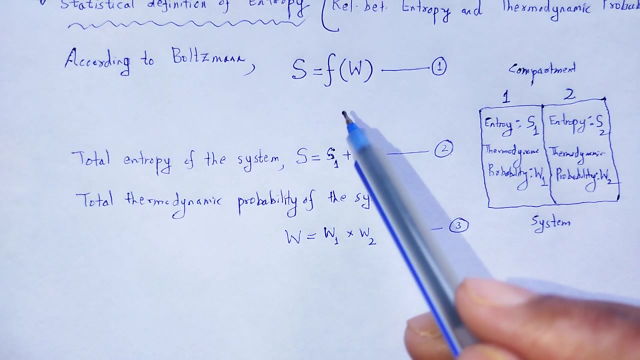 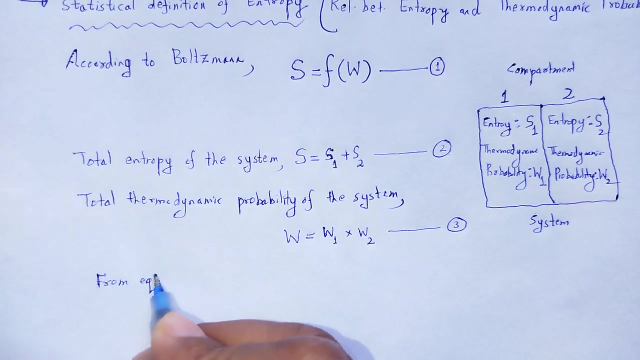 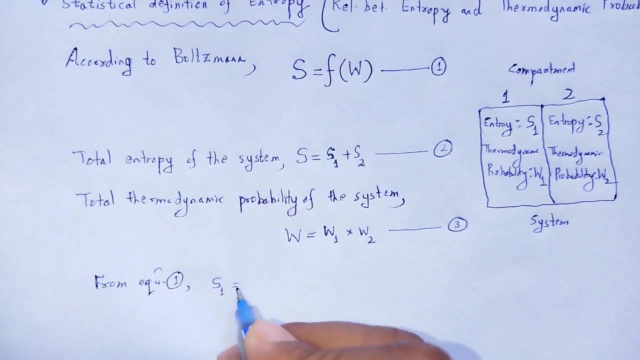 to the product of individual thermodynamic probability of the compartments, that is W 1 into W 2, equation number 3.. Now we can use equation number 1 as a entropy is a function of thermodynamic probability. So equation number 1, we write from equation number 1, S 1 is the function of W 1, equation. 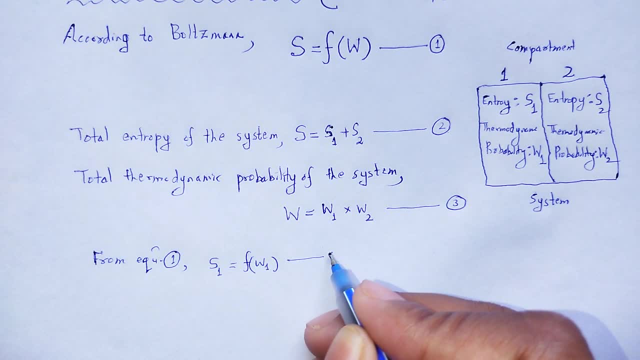 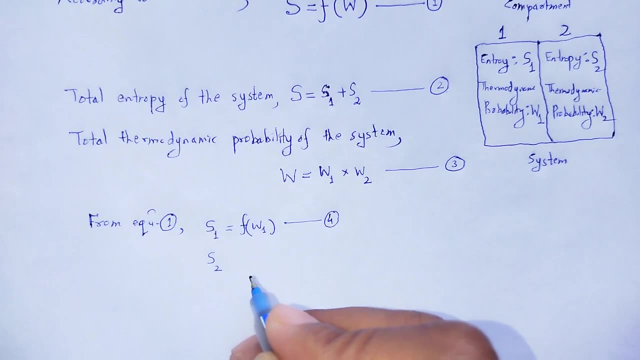 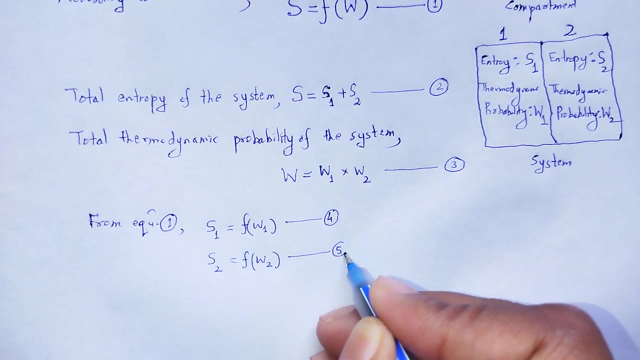 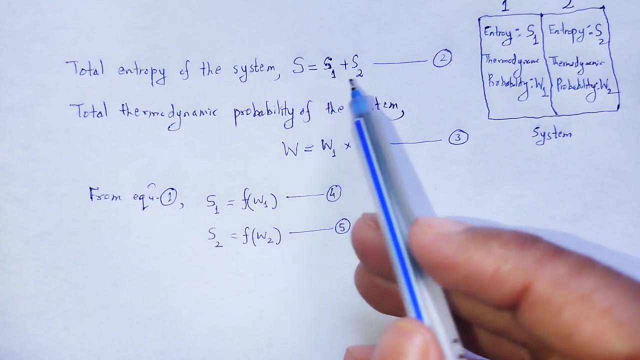 number 3, S 2 is the function of W 2, equation number 3.. And then S 1 is a function of W 2, equation number 3.. And from equation number 3, S 2 is a function of S 1.. Now S 1 is a. 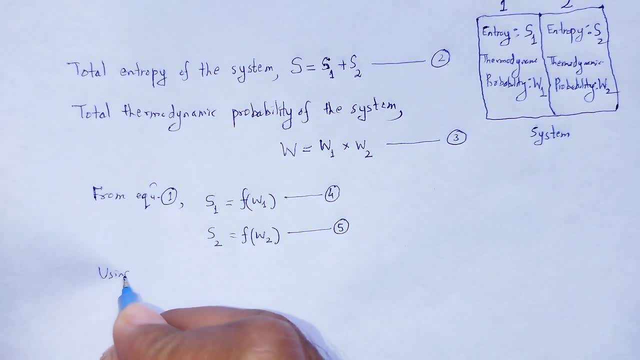 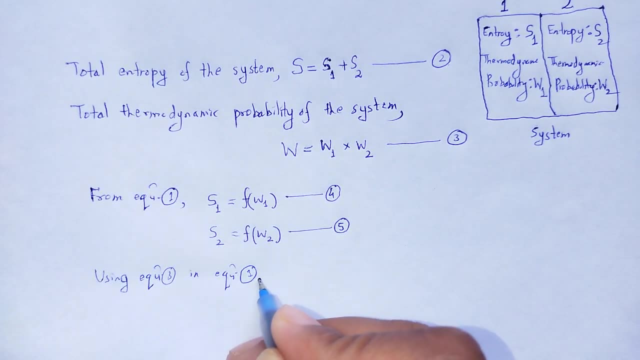 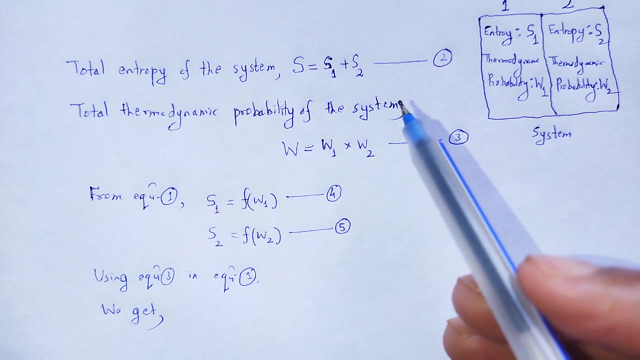 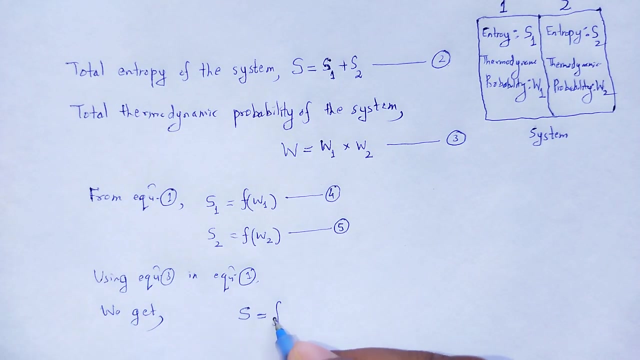 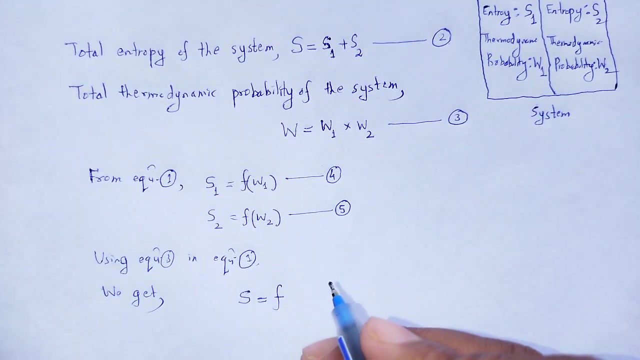 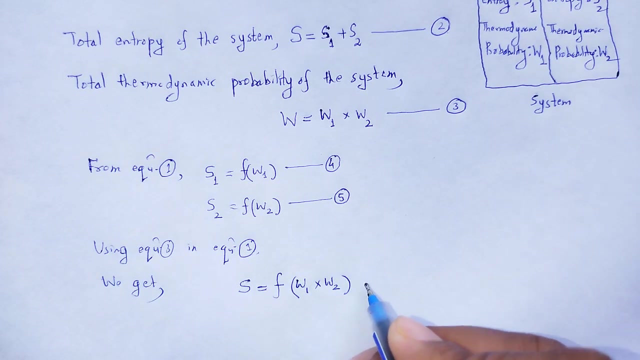 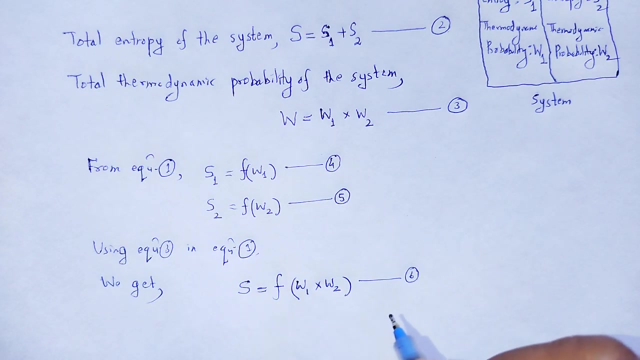 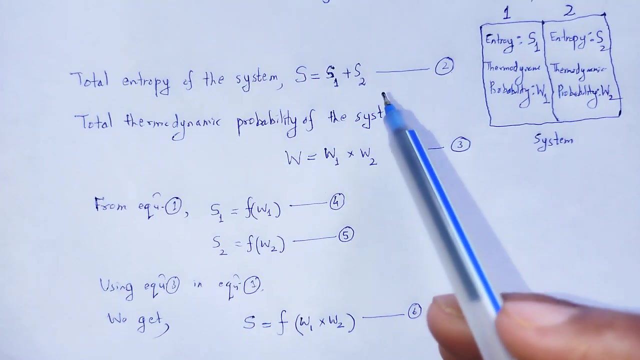 1 using equation number 3, in equation number 1 we get: S is equal to function of w in place of w. product of w 1 into w 2, w 1 into w 2 in equation number 3.. Now equation 2 can be written as we put. 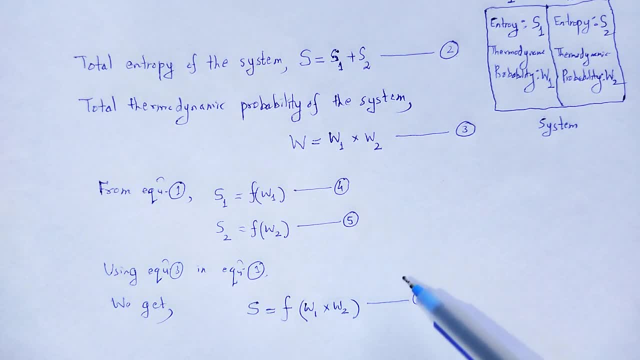 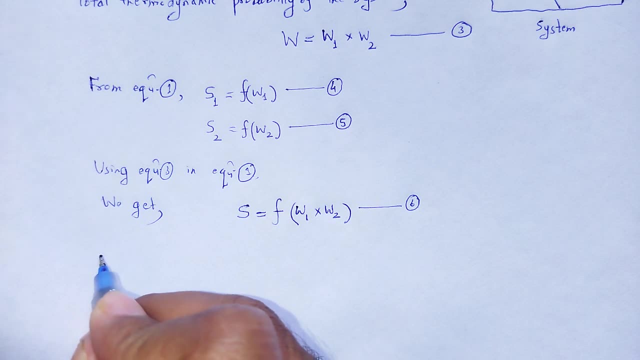 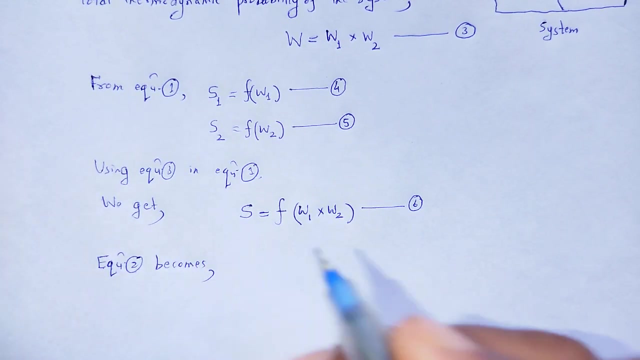 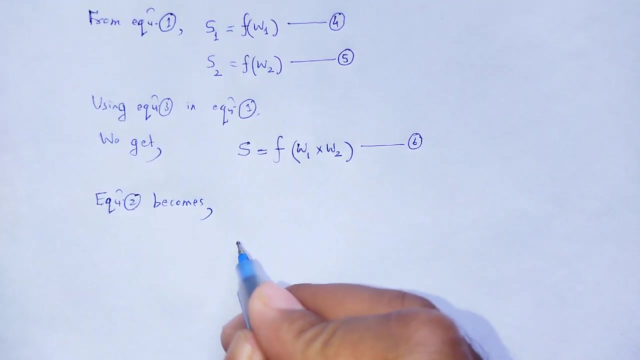 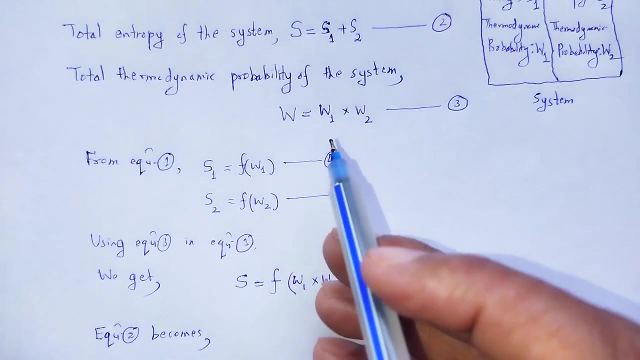 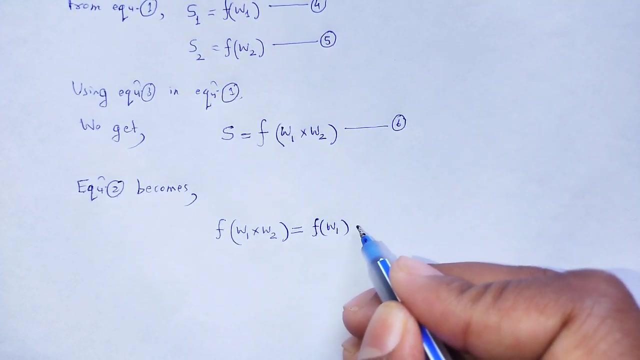 s1 by s2 function of w 1 plus s2 function of w 2, the equation number: 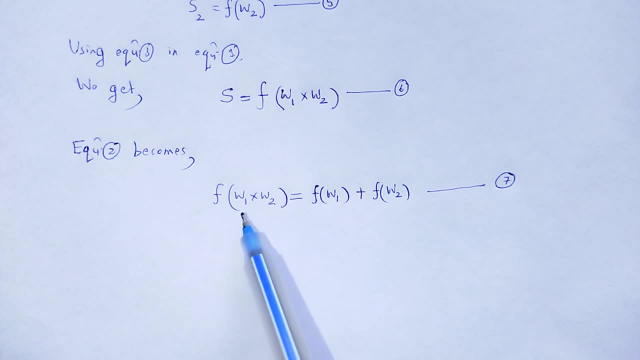 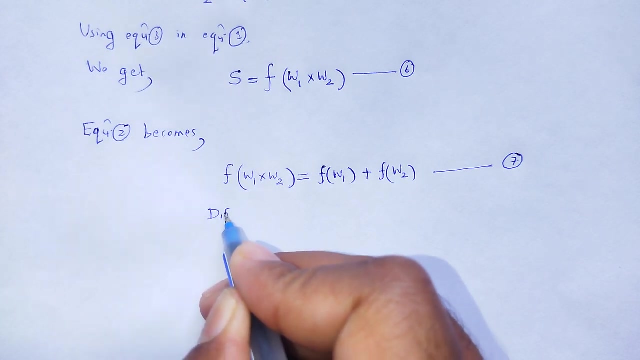 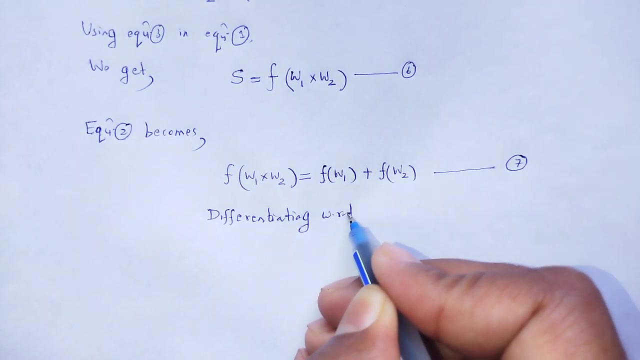 7. As it has 2 variables, one is w 1 and another one is w 2, so we differentiate it with respect to w 1- this is w 1. 1- and also with respect to w 2.. First, we differentiating it, differentiating, differentiating with respect. 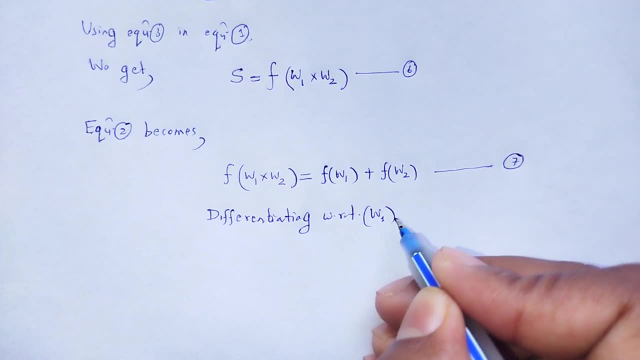 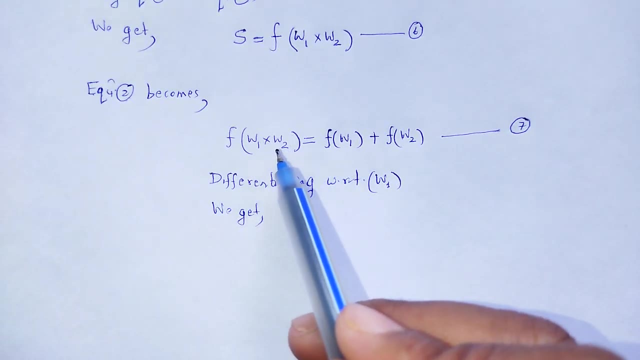 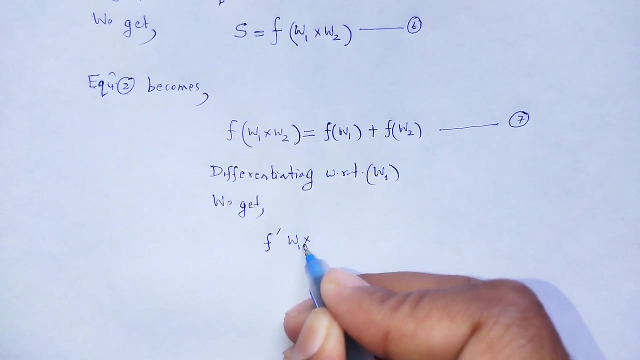 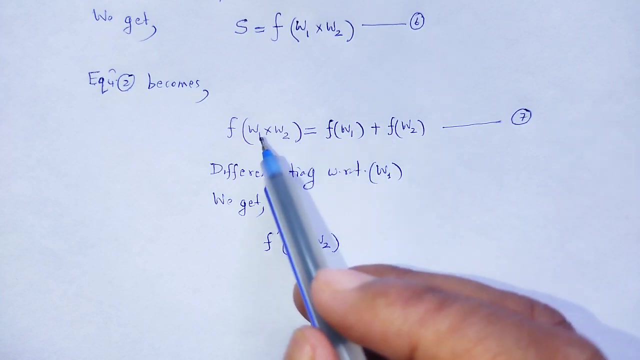 to w 1, we get. this is the product of w 1 into w 2, and this first order differentiation f dash w 1 into w 2, then as we differentiate with respect to w 1.. So w 2 as constant w. 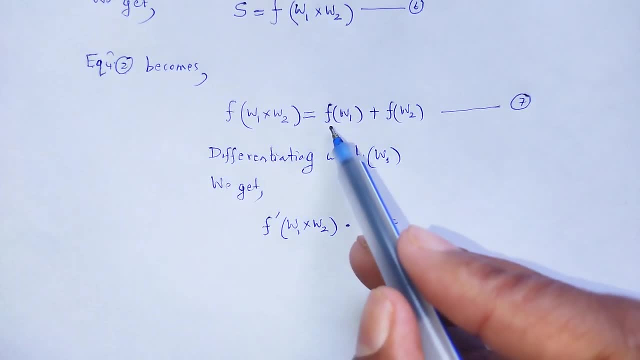 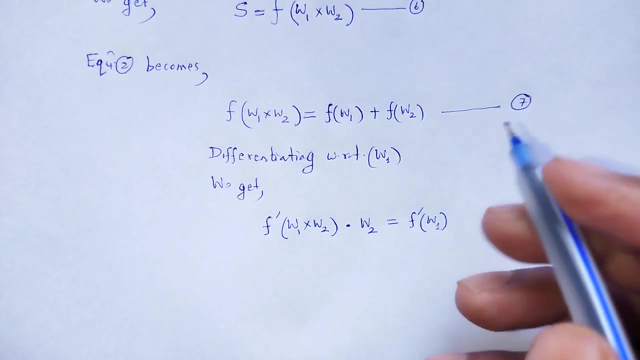 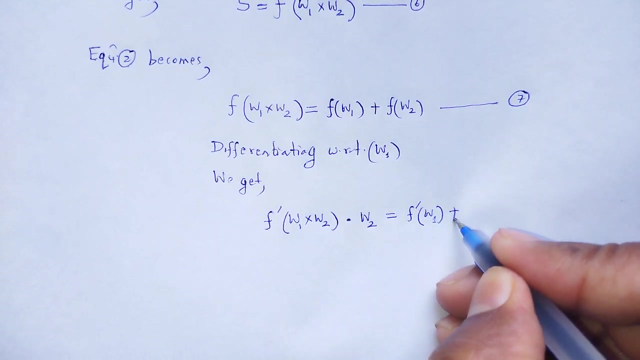 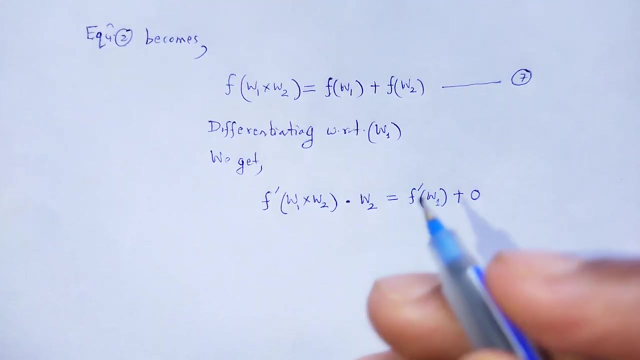 2.. Next, w 1 is equal to f of w 1. that is first order differentiation of w 1.. Next, w 1 with respect to w 1, derivative as 1 plus f of w 2 with respect to w 1. results 0, rewrite f. 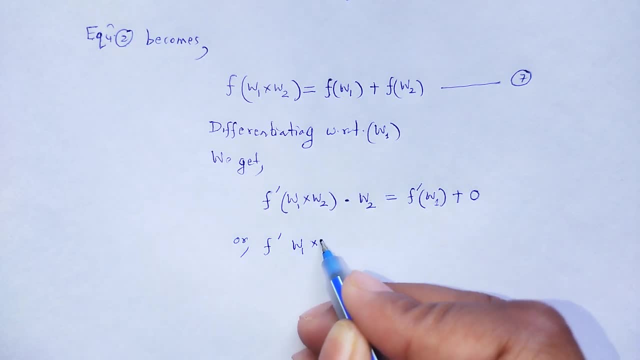 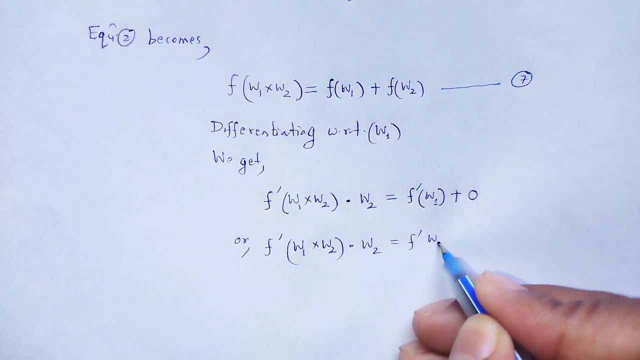 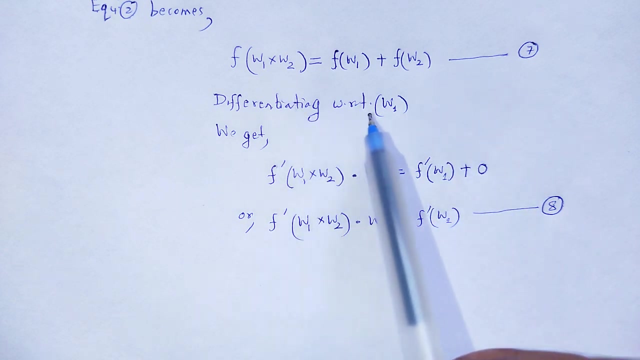 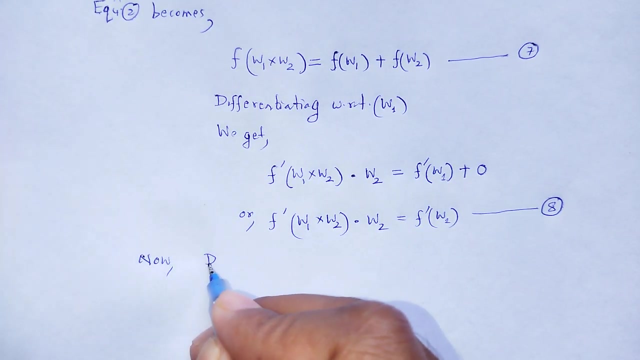 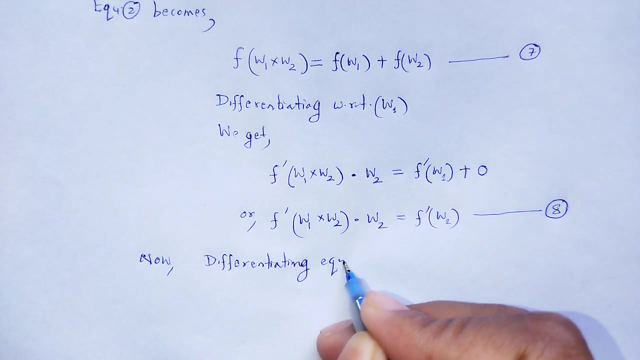 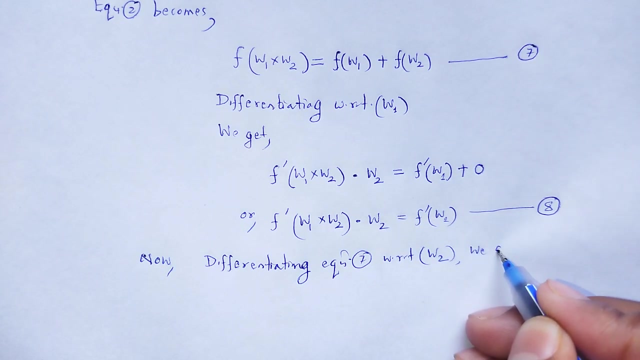 dash 2 into w 2 into w 2 is equal to f dash w n, the equation number 8.. Now, differentiating that equation number 7 with respect to w 2, now differentiating equation number 7 with respect to w 2, we get: 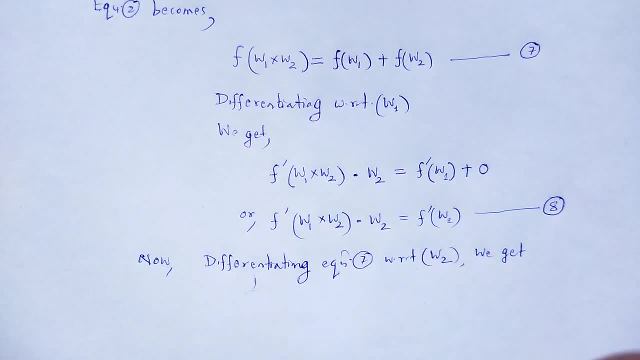 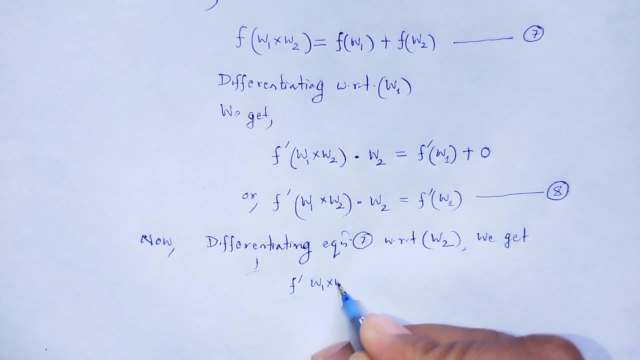 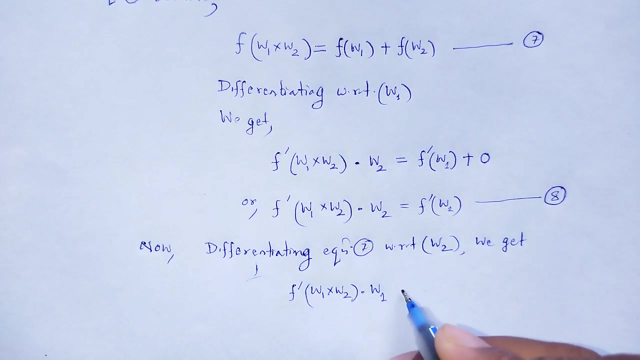 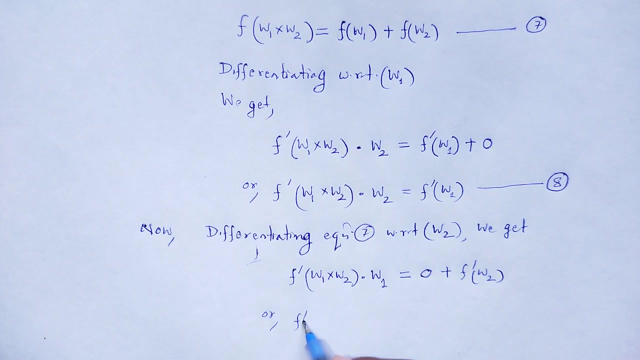 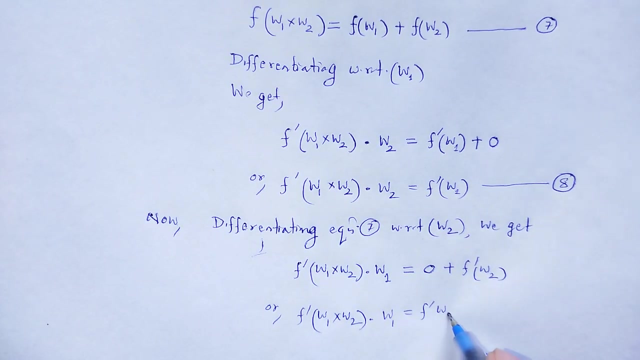 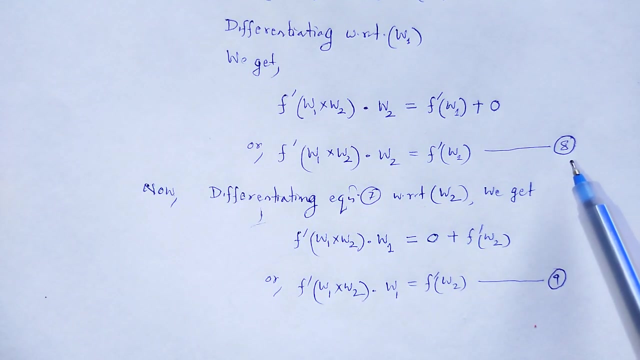 First word: differentiation f dash w 1 into w 2, as we differentiate with respect to w 2.. So it has: w 1 is equal to differentiation with respect to w 2. results 0 plus f dash w 2 or f dash w 1, w 2: w 1 is equal to f dash w 2. equation number 9.. Now we divide equation. 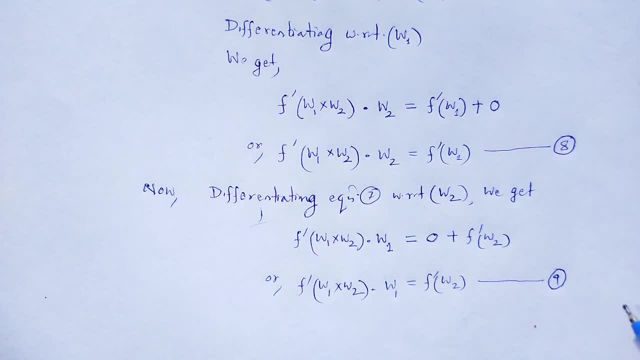 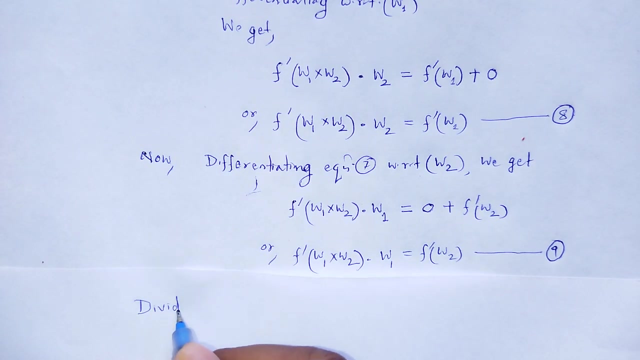 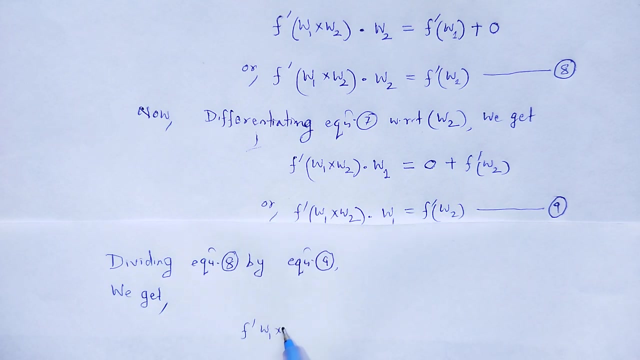 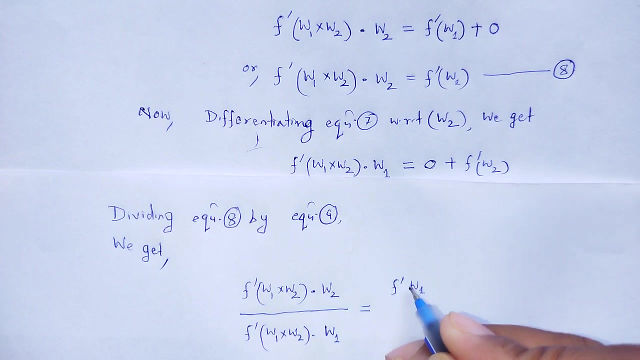 number 8 by equation number 9.. So by dividing equation number 8 by equation number 9, we get equation number 8 as f dash w 1 into w 2.. So f dash w 1 into w 2, divided by f dash w 1 into w 2 into w 1, is equal to f dash w.